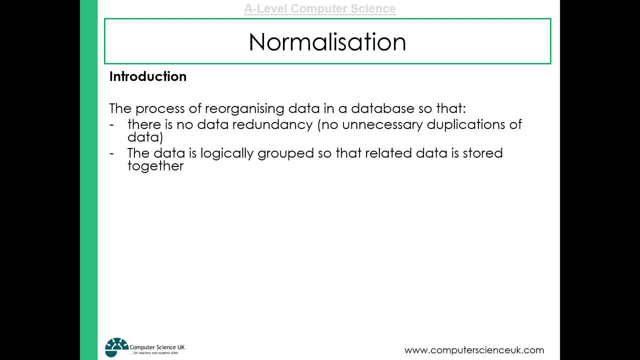 really logically grouped by entity. Okay, so normalization is a process of making sure that these issues don't happen. Now, in order to do normalization, we we go through three stages. So first, normal form, second, normal form and third, normal form, and the whole point of this is so that 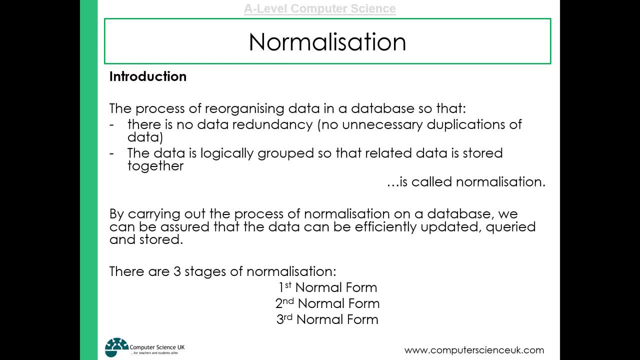 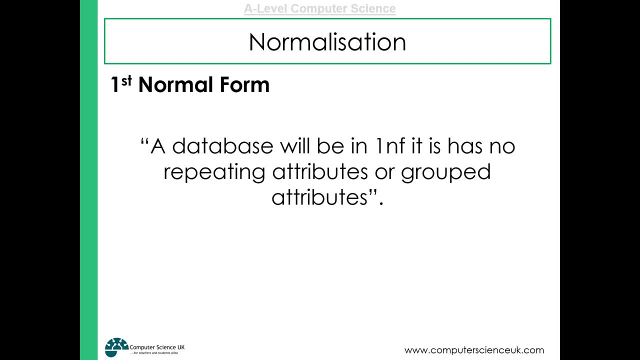 we can be sure that data can be efficiently updated, queried and stored. So let's have a look at first normal form. So first normal form is a process of making sure that data can be stored. So the rule for first normal form is that the database will be in first normal form if it 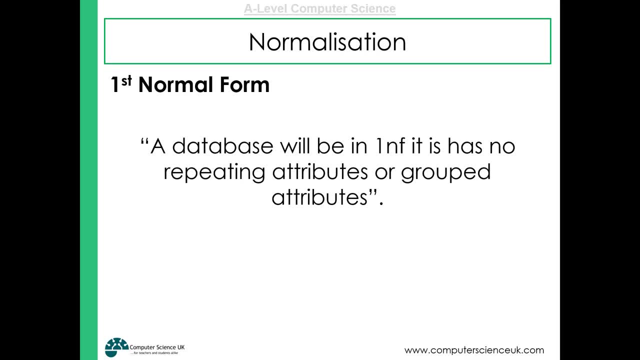 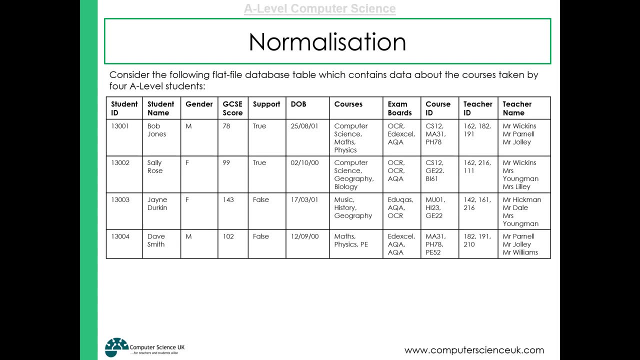 has no repeating attributes or grouped attribute attributes, sorry. So if you consider this flat file database table and what it is doing is it's showing several students- a-level students- and the courses that they're enrolled in, their exam boards and their teachers. So if you look, 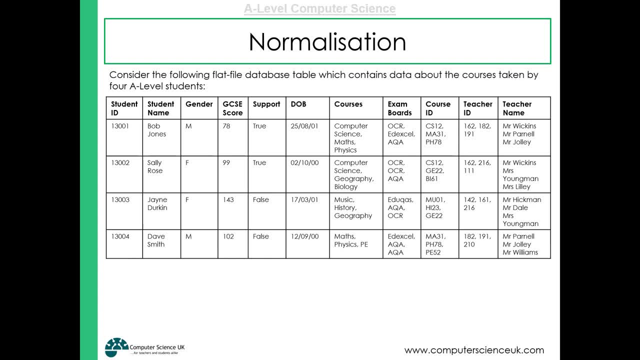 at a row, for example, Bob Jones, the first row- we've got information about that student: their gender, their GCSE score, whether they have support or not, their date of birth, and then we've got the courses that they are enrolled in, the exam boards for each of those courses and also the teachers. 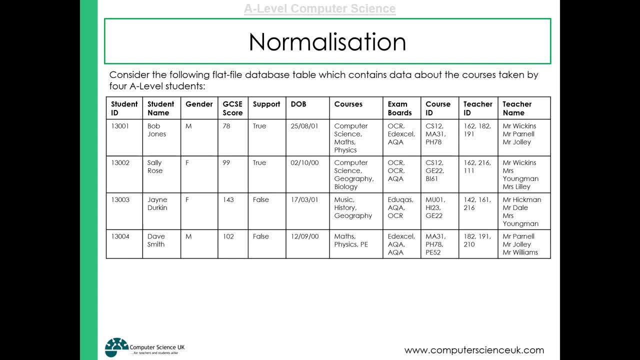 which take those courses, which run those courses or lead them. Now we've got several fields here where we've got grouped attributes. So we've got courses, exam boards, teacher name. these have all got grouped attributes. and the problem with having grouped attributes is that we can't actually 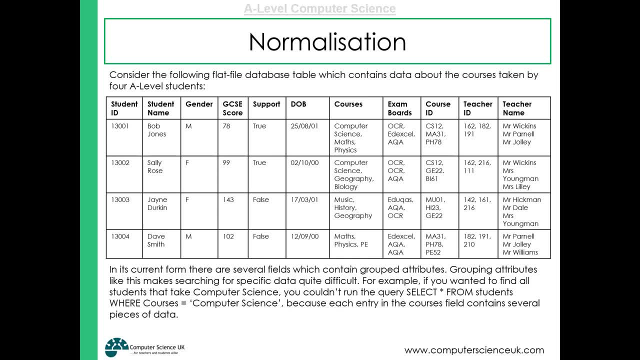 search for particular bits of data. we can't query our database that easily. For example, if we wanted to find all the students that took computer science, we couldn't run an SQL statement of select everything from students where courses equals computer science, Because each entry in the courses field contains several pieces of data. 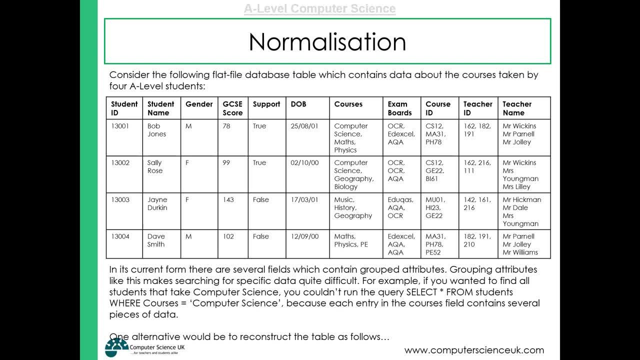 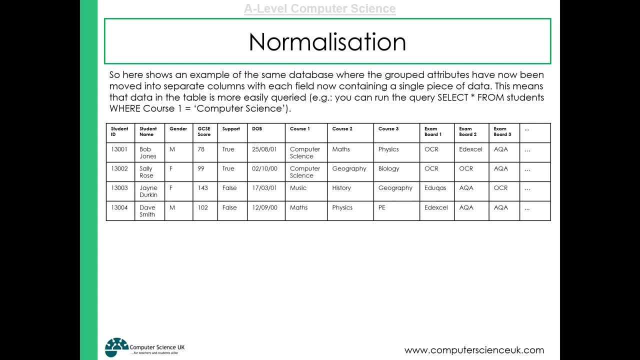 So what we could do is we could reconstruct this table to ensure that we don't have any grouped attributes. So you can see here how we have now got each row for each student, but instead of having grouped attributes, we've actually split the different courses up so that we've 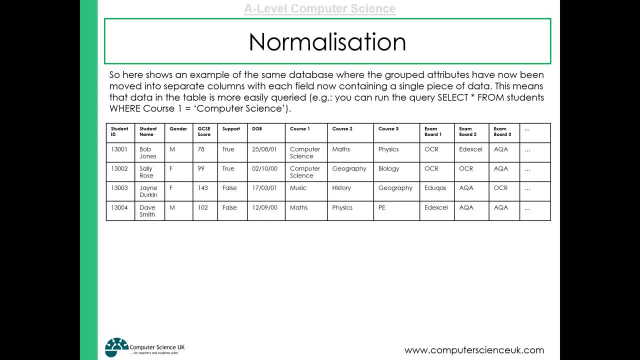 got course one, course two and course three, The same for the exam boards, and if I had space I would have carried that on for teachers as well. So now we could, if we wanted, to do a query and to find out whether a student was doing computer. 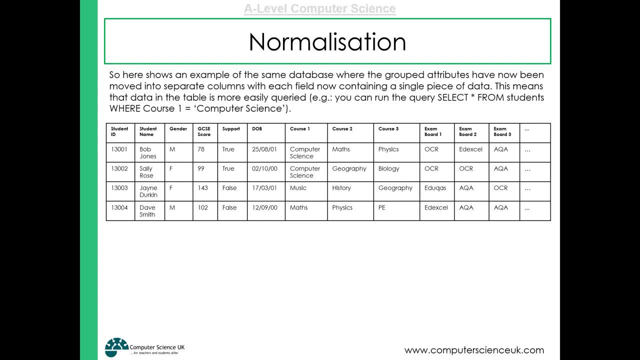 science, for example, Although we would need to run that in several courses columns. Now we've still got an issue here because in its current form we've actually got repeated attributes. Okay, they're not grouped anymore, but they are repeated attributes: Course one, course two, course three, they're all repeated. 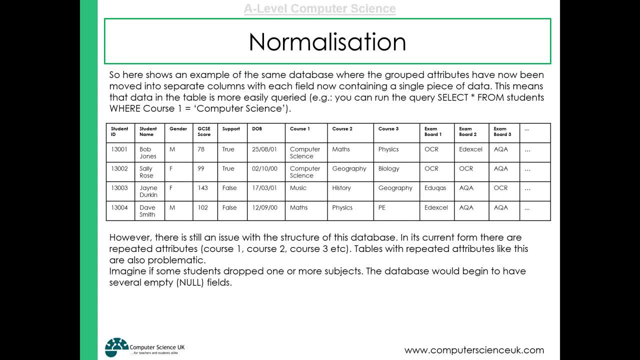 And that does bring some problems. So imagine if a student wanted to drop a subject. the database would begin to have null fields, so it's empty fields. And if a student wanted to, you know, enrol on another course, a fourth course would have to. 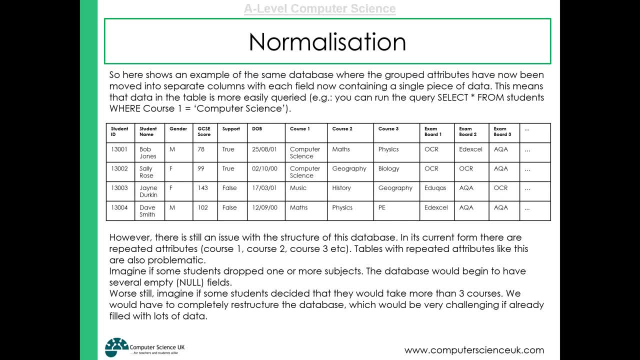 completely reconstruct this database table in order to actually allow that to be stored, And that could be very problematic indeed. So the process of normalisation seeks to solve all these issues And we're now going to have a little look to see how we can actually 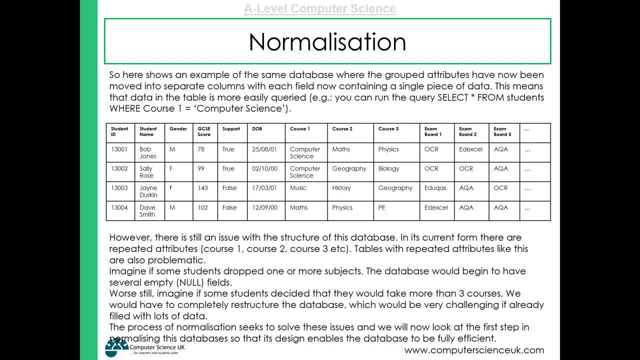 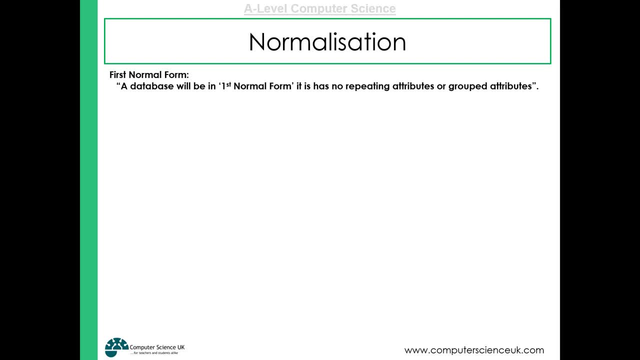 run normal, go through the steps of normalisation so it can be as efficient as possible. So remember: first normal form. a database will be in first normal form if it has no repeating attributes or grouped attributes. So we've seen an example of repeated attributes. we've changed. 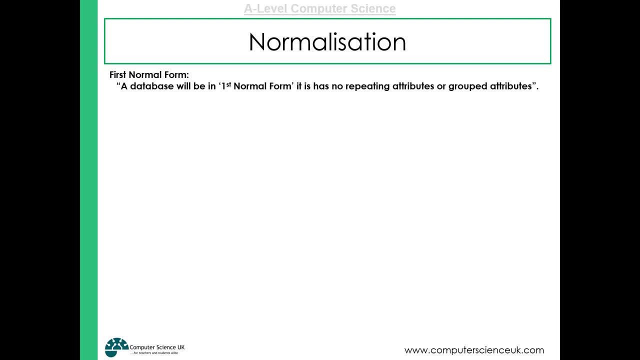 the table, so it's got sorry. we've had an example of a table with grouped attributes. we've changed that structure so it had repeated attributes. But if we want to get our previous database table into first normal form, we simply need to just increase the number of records that it has. so 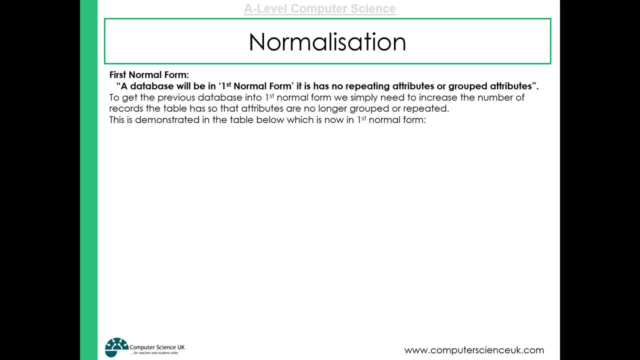 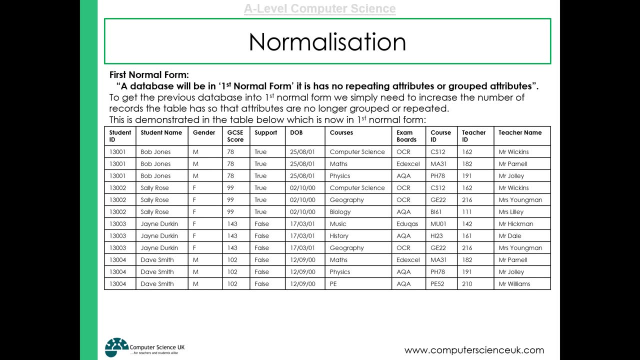 the attributes are no longer repeated. So here's an example. You can see now that we haven't got three columns for courses, we haven't got three columns for exam boards or for teachers. we've simply got a single attribute: courses, Same for exam boards and teacher name. But what we've done for each student is we've actually got 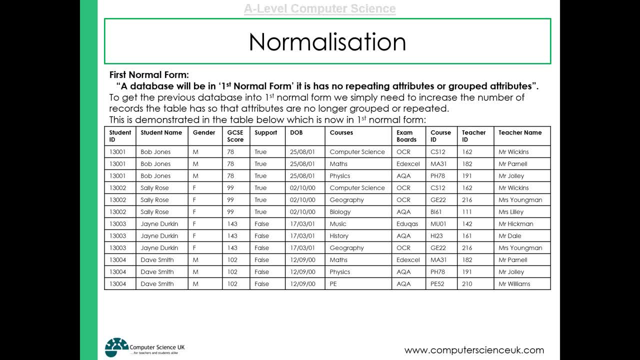 several records for each student. So Bob Jones is now on three different rows, three different records, And each record it shows the course that he's enrolled in, the exam board that goes with that course and the teacher of that course. So this table can now be easily queried. Each. 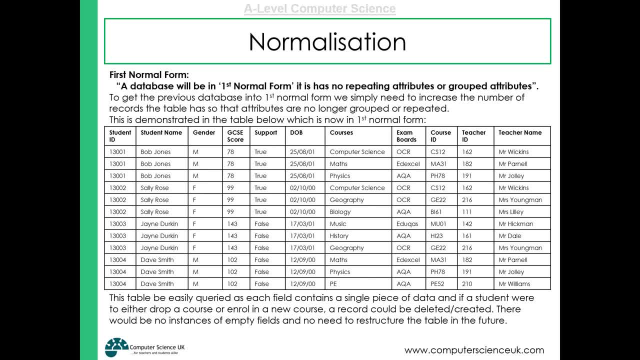 field contains a single piece of data, And if a student were to either drop a course or enrol in a new course, we'd just simply delete or create a record, So there'd be no instances of empty fields. we wouldn't need to reconstruct the table in the 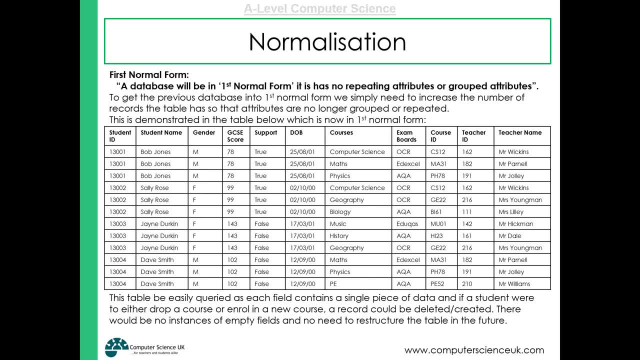 future. So this is an example of a database in first normal form, But it's not perfect. Okay, there's still lots of repeated data, lots of redundant data redundancy. So they've got the same data stored more than in more than one place in the data. 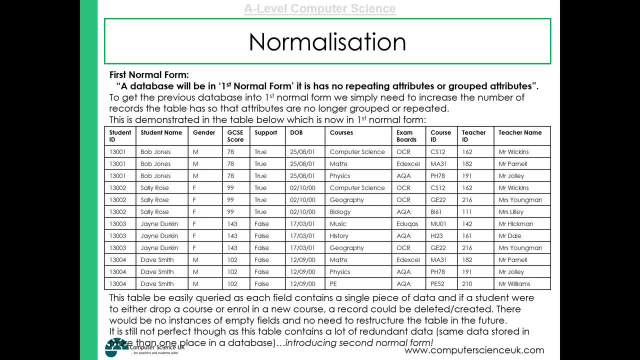 database. So we've gone into first normal form. it's now time to see if we can go into second normal form. Now, just to sort of put this into into sort of an example that we've seen before, if you look at the or think about the video that we had previously where we were looking at 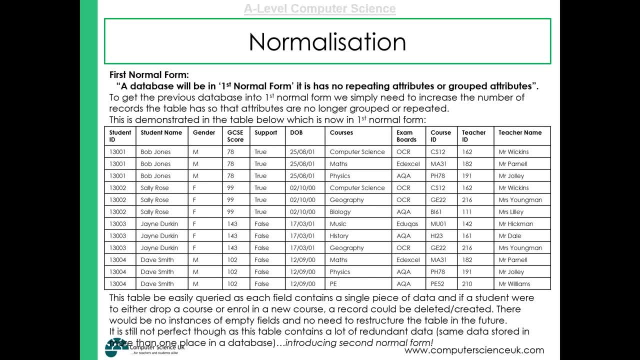 relational databases. we had a look to a database for a shop And by splitting that database up into several tables and then linking them together, That is the process of going into second and potentially third normal form. So we've got a flat file database here. It's okay, we can query it, but it is not that efficient. 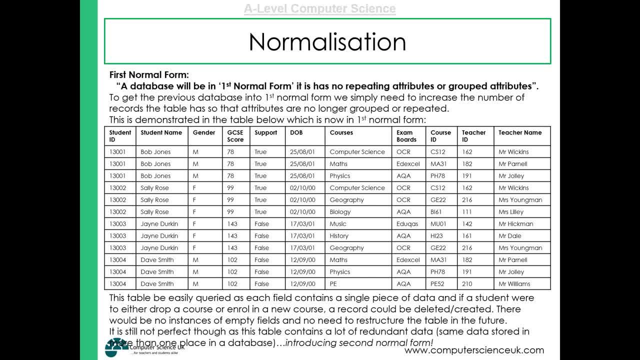 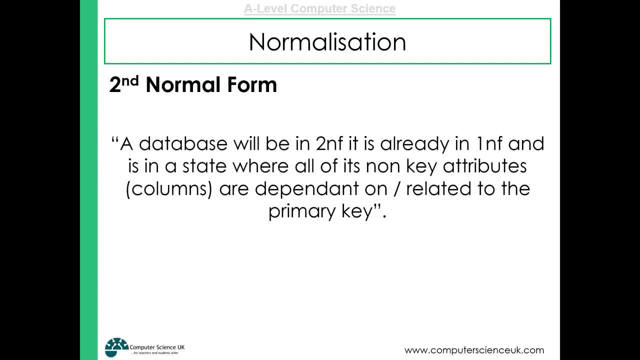 So let's have a look at how we can turn this database into a more efficient one by going into second normal form. So second normal form is where a database is already in first normal form and is also in a state where all of key attributes are dependent on or related to the primary key. now that 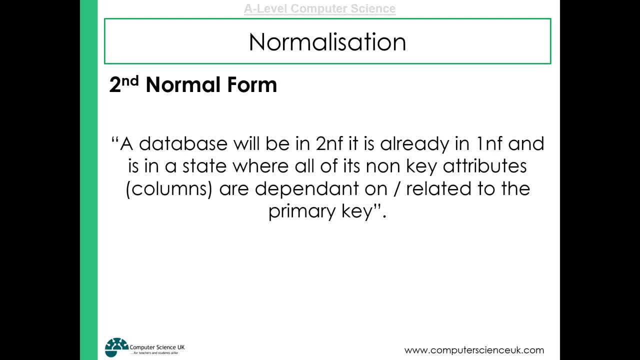 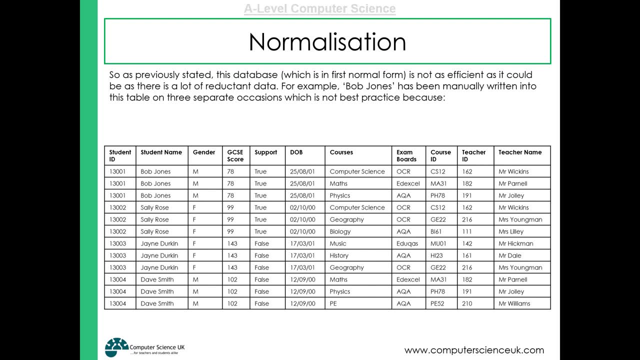 sounds really confusing. so the best way to get around this is to have a little look at an example. so we're back to our table that we we looked at before. so this table, as we know already, it's in first normal form. it's not as efficient. 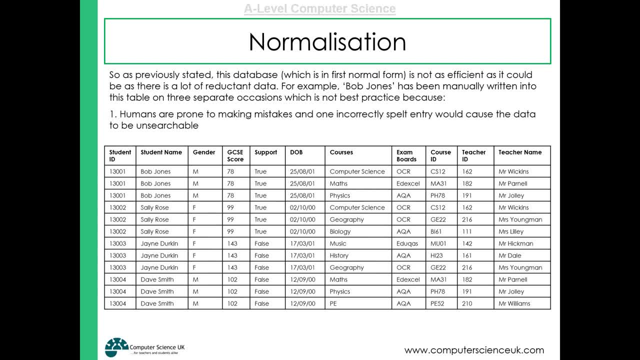 as it could be. and the reason why it's not efficient is that Bob Jones has to be manually written into this table on three separate occasions, or Sally Rose does, or Jane Durkin and so on, and the reason why it's not good to have this duplication of data, as we sort of discussed in the previous lesson- humans. 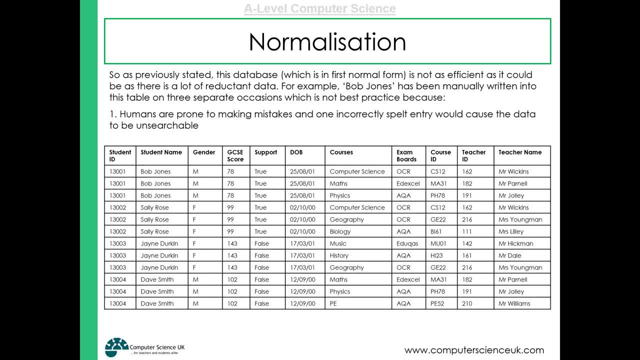 are prone to making mistakes, and if you incorrectly spell an entry somewhere in the database, it will be unsearchable. more storage is required to store the duplicated data as well. not great. so to overcome this problem, we can split the table into two parts. and we can split the table into two parts, and we can split. 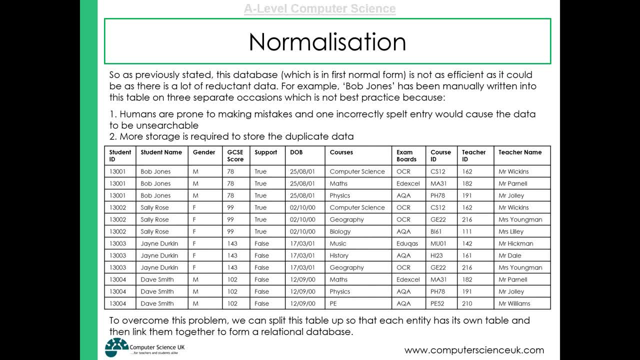 the table into two parts and we can split the table up so that each entity has its up, so that each entity has its own table, and then we can link them together. so we own table and then we can link them together. so we said before, this sort of 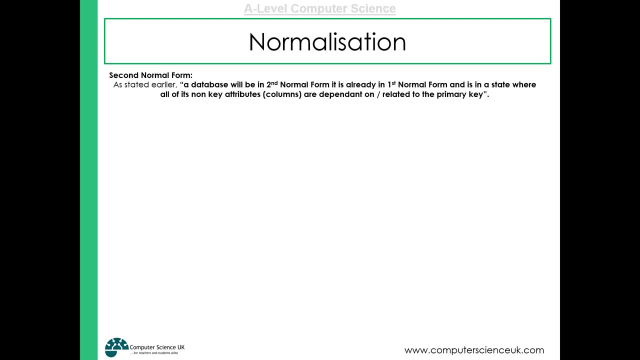 said before this sort of confusing statement. a database will be in. second confusing statement. a database will be in second normal form if it's already in normal form, if it's already in first normal form and is in a state where all first normal form and is in a state where all of its non key attributes are. 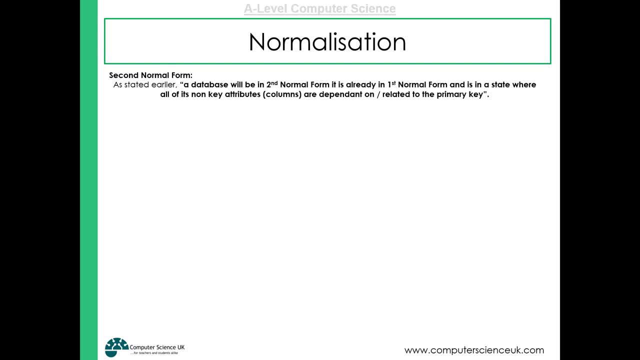 of its non key attributes are dependent on or related to the primary key. what dependent on or related to the primary key? what we're talking about there is? we're talking about there is that each table has to hold data about a single, that each table has to hold data about a single entity. so the 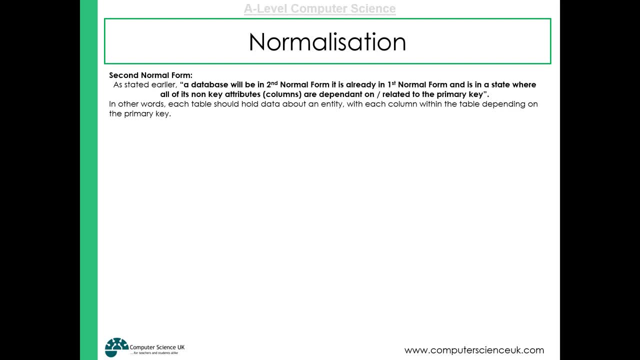 entity. so the attributes of the table should all depend or relate to. the attributes of the table should all depend or relate to the primary key, the entity itself. so each primary key, the entity itself. so each column within the table should depend on. column within the table should depend on the primary key. each table should be: 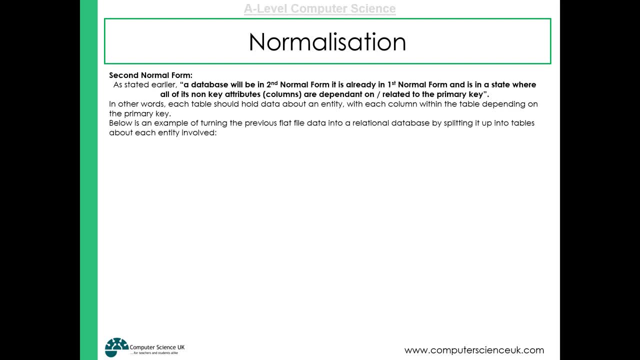 the primary key. each table should be about an entity. so what we're going to about an entity, so what we're going to see now is an example of turning the see now is an example of turning the previous flat file database into a previous flat file database, into a relational database. so it's in. second, 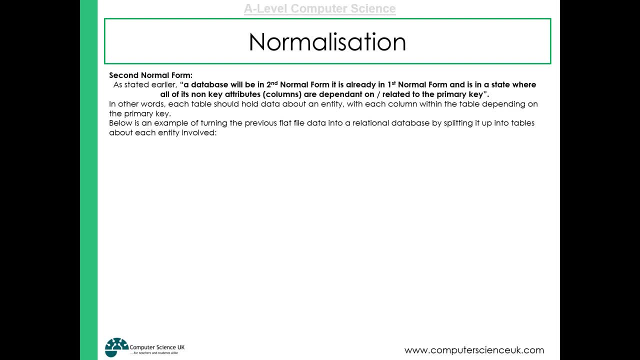 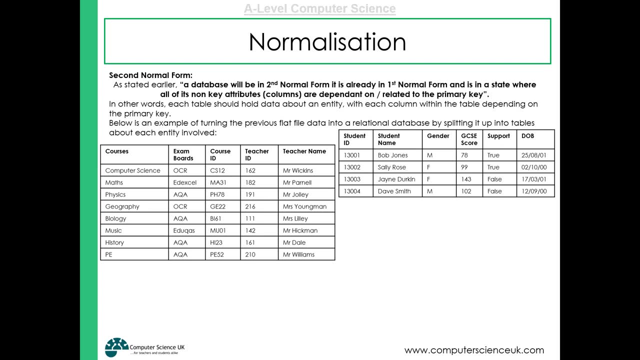 relational database. so it's in second normal form by splitting up the splitting normal form by splitting up the. splitting it up into tables about each. it up into tables about each entity, it up into tables about each entity. so here we've got an example of a table. 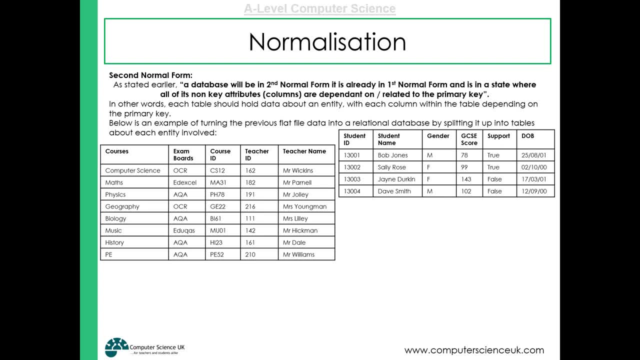 so here we've got an example of a table just about the students, and you could just about the students and you could see here that each student has its name. see here that each student has its name, gender GCSE score support, that it has gender GCSE score support, that it has date of birth, and that information definitely does. 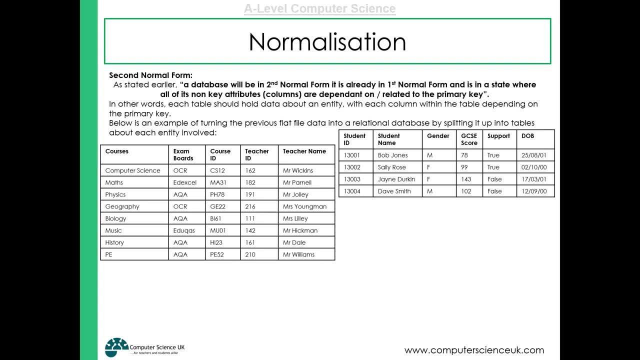 date of birth and that information definitely does relate to the student. we've got relate to the student, we've got courses here, the different courses that are run, courses here, the different courses that are run at a level, their exam boards and the at a level, their exam boards and the teachers that run it. so, on the face of 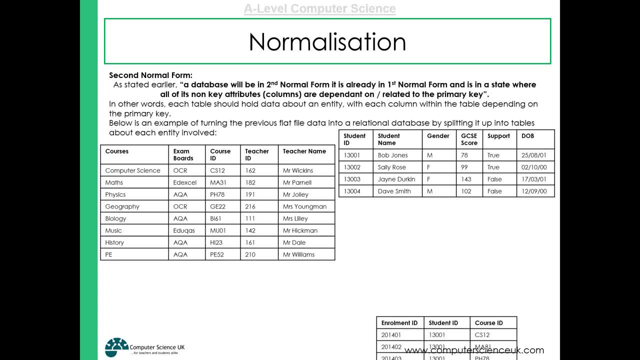 teachers that run it. so on the face of it looks like that all relates to the. it looks like that all relates to the course. so we sort of split it up into course. so we sort of split it up into two tables, and then we could have this: 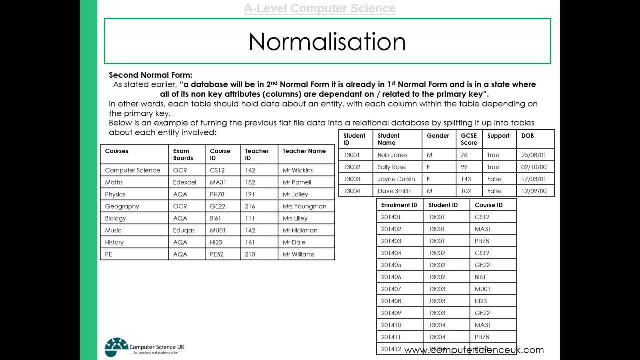 two tables and then we could have this sort of intersecting table where we can sort of intersecting table, where we can start to link them, link them up, so each start to link them, link them up, so each enrollment- for example a student going enrollment, for example a student going into a course, is an enrollment we could. 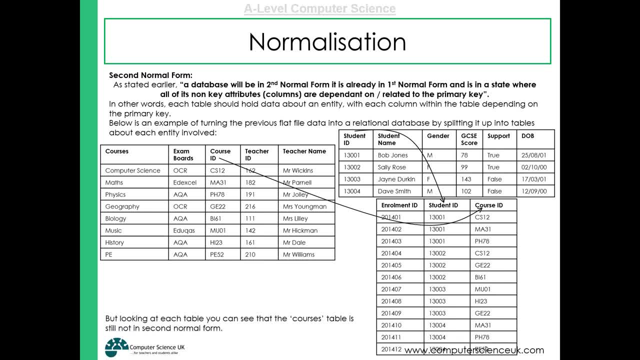 into a course is an enrollment. we could have an enrollments table now. if you have an enrollments table now, if you actually study the courses table in a, actually study the courses table in a bit more detail, you can see it's still bit more detail. you can see it's still not in second normal form you could have. 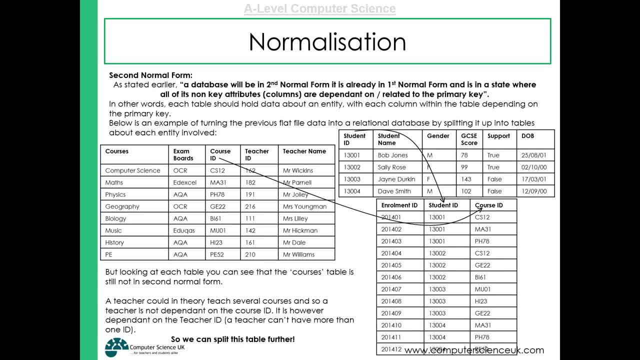 not in second normal form. you could have a situation where a teacher teaches more, a situation where a teacher teaches more than one course. so therefore, than one course, so therefore, than one course. so therefore, a teacher isn't dependent on the course and a teacher isn't dependent on the course. and 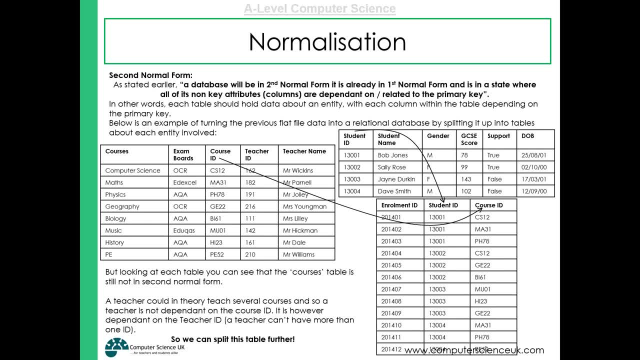 a teacher isn't dependent on the course and because of that, we need to split this. because of that, we need to split this. because of that we need to split this table up even further. if we want to get table up even further, if we want to get. 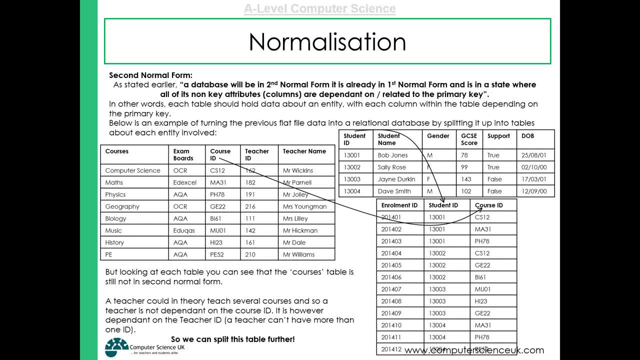 table up even further if we want to get it into true second normal form, so a it into true second normal form. so a it into true second normal form. so a teacher is actually only really teacher, is actually only really teacher, is actually only really dependent on its ID. it's not necessarily. 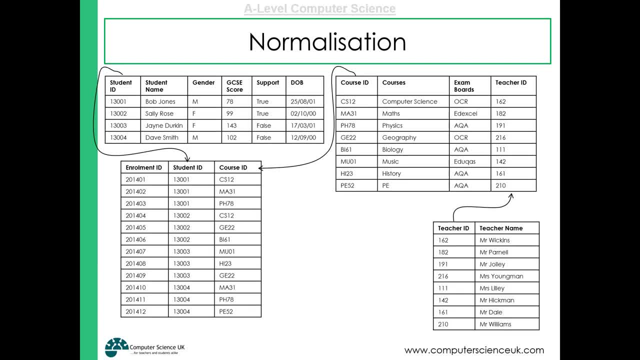 dependent on its ID. it's not necessarily dependent on its ID, it's not necessarily dependent on the course. so let's split. dependent on the course. so let's split. dependent on the course. so let's split it up even further. so now we've got an it up even further. so now we've got an. 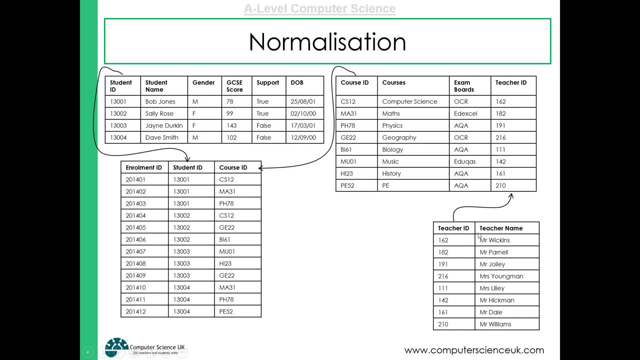 it up even further. so now we've got an our teachers table because now that our teachers table, because now that our teachers table, because now that we've got our teacher teachers separated, we've got our teacher teachers separated. we've got our teacher teachers separated if a teacher was to teach more than one. 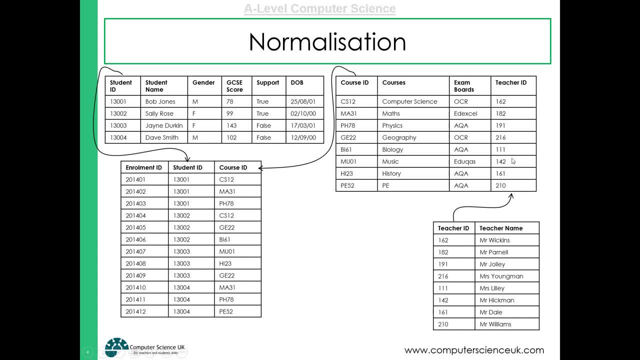 if a teacher was to teach more than one. if a teacher was to teach more than one course, then their ID could be placed in course. then their ID could be placed in course. then their ID could be placed in the appropriate record. much better doing. the appropriate record. much better doing. 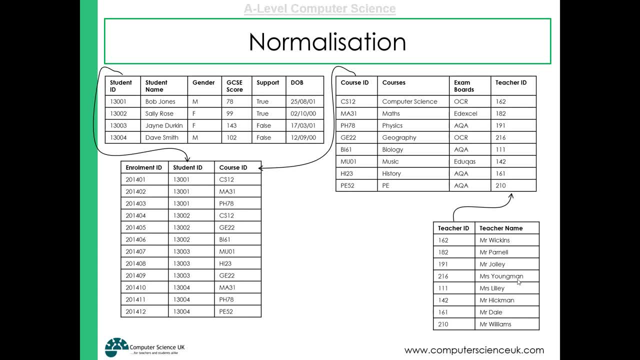 the appropriate record. much better doing it that way than having to repeat it that way, than having to repeat it that way, than having to repeat teachers names over and over again. so if teachers names over and over again, so if teachers names over and over again, so if we want to go to second normal form, 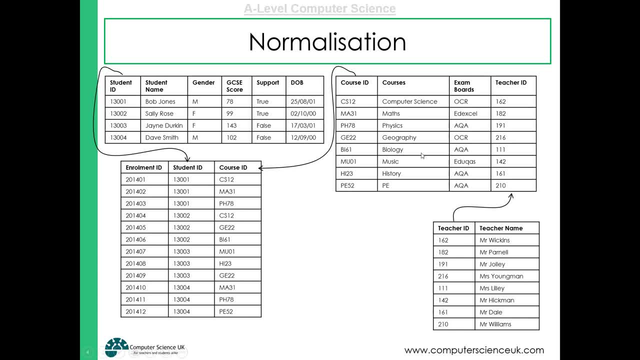 we want to go to second normal form. we want to go to second normal form. it's about all of the attributes in each. it's about all of the attributes in each. it's about all of the attributes in each table, depending only on the primary key table, depending only on the primary key. 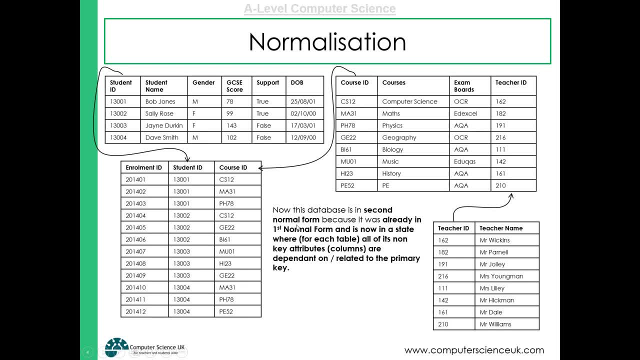 table depending only on the primary key. so this database is in second normal. so this database is in second normal. so this database is in second normal form because it was already in first form, because it was already in first form, because it was already in first normal form and is now in a state where 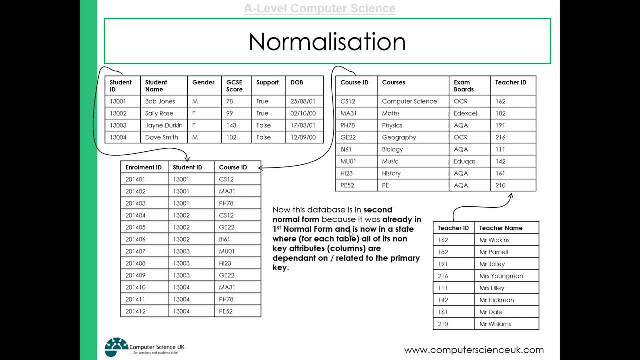 normal form and is now in a state where normal form and is now in a state where, for each table, all of its non key, for each table, all of its non key. for each table, all of its non key attributes, all of its columns are attributes, all of its columns are. 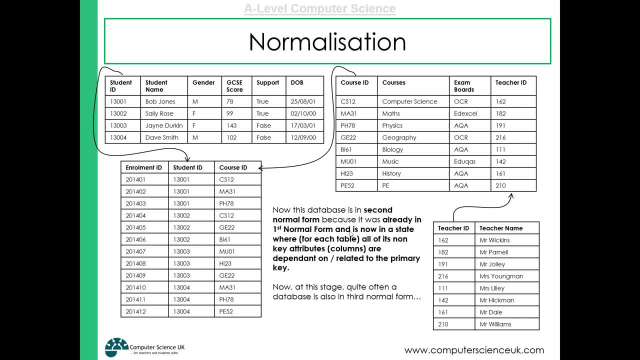 attributes: all of its columns are dependent on or related to the primary, dependent on or related to the primary, dependent on or related to the primary key, and usually at this stage when we go key, and usually at this stage when we go key, and usually at this stage when we go through the process of normalization. 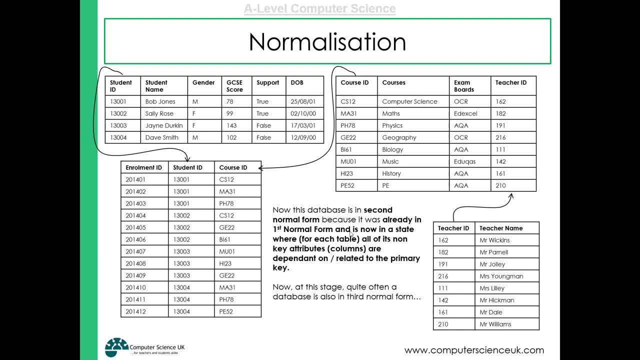 through the process of normalization. through the process of normalization, it's often, always, or often also in third. it's often always, or often also in third. it's often, always, or often also in third normal form. but we do always have to normal form, but we do always have to. 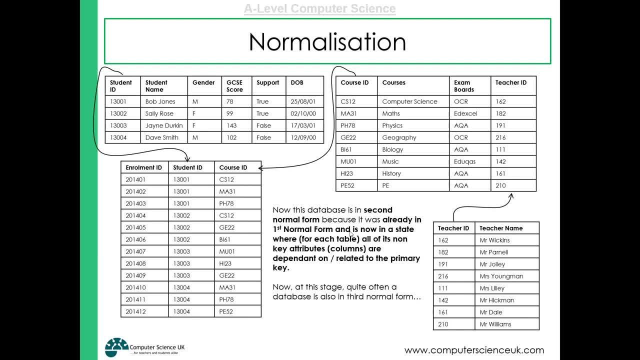 normal form. but we do always have to check, and that's really important check, and that's really important check and that's really important, certainly in an exam, well, obviously in. certainly in an exam, well, obviously in. certainly in an exam, well, obviously, in real life it's important, but in the exam 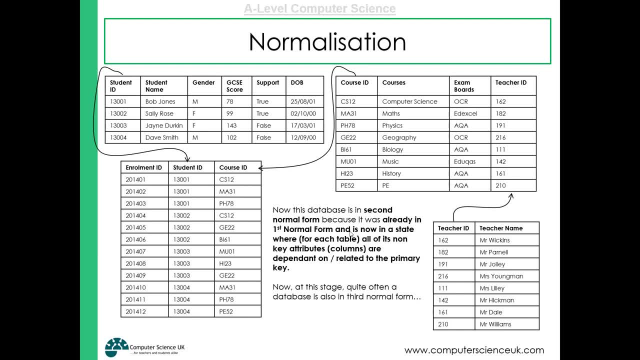 real life it's important, but in the exam, real life it's important, but in the exam, it might be you get to this point, and it might be you get to this point and it might be you get to this point and you just need to do a double, double. 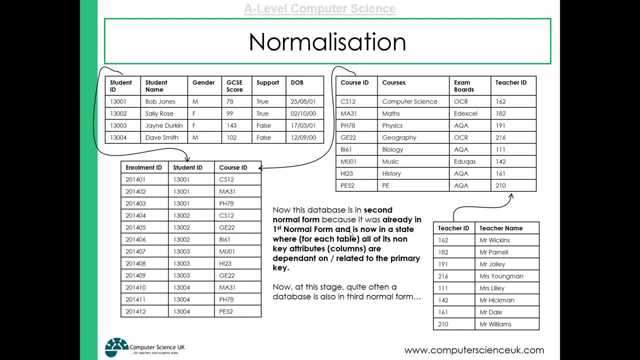 you just need to do a double double. you just need to do a double double check to see if it's also in third check, to see if it's also in third check, to see if it's also in third normal form. so what is third normal form? 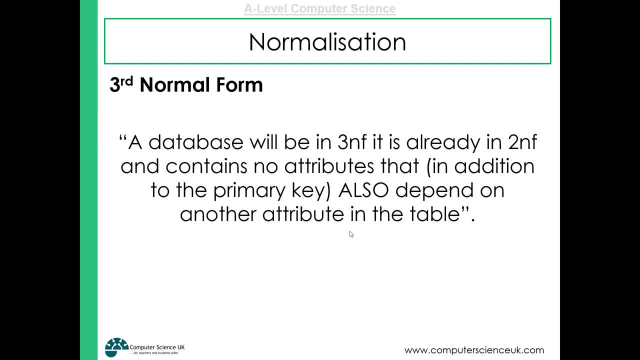 normal form. so what is third normal form? normal form, so what is third normal form? third normal form is where a database is. third normal form is where a database is third normal form is where a database is already in second normal form and already in second normal form, and 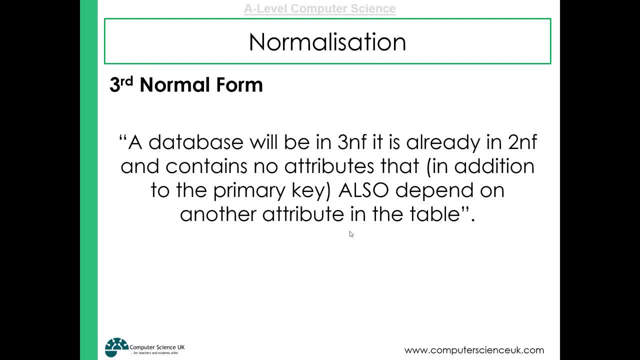 already in second normal form and contains no attributes. that, in addition, contains no attributes. that, in addition, contains no attributes. that, in addition to the primary key, also depend on to the primary key, also depend on to the primary key, also depend on another attribute in the table again. 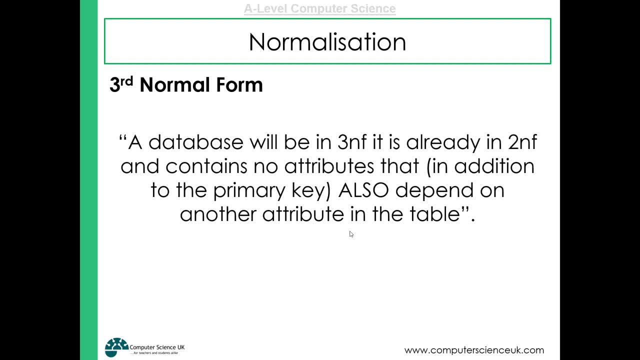 another attribute in the table. again another attribute in the table, again confusing. so let's see if we can see an confusing. so let's see if we can see an confusing. so let's see if we can see an example of what this actually means and example of what this actually means. and 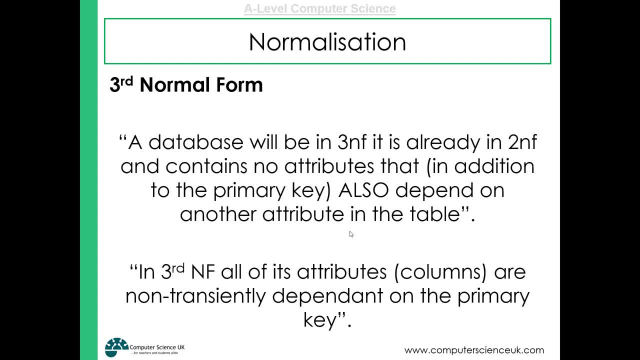 example of what this actually means. and here's another definition, which is: here's another definition, which is: here's another definition which is probably a little bit more confusing in: probably a little bit more confusing in, probably a little bit more confusing in third normal form, all of its attributes. 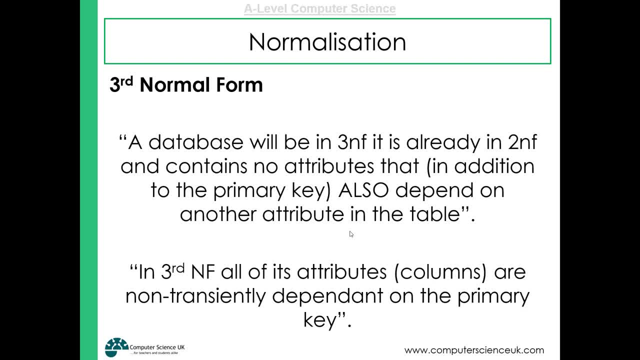 third normal form: all of its attributes. third normal form, all of its attributes are non transiently dependent on the are non transiently dependent on the. are non transiently dependent on the primary key. let's see if we can. primary key. let's see if we can. 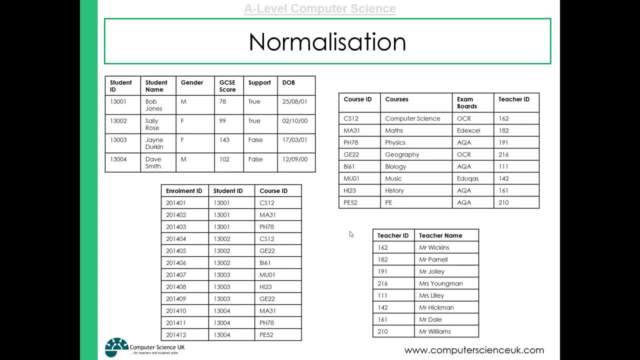 primary key. let's see if we can understand what that means. so we've got understand what that means. so we've got understand what that means. so we've got our tables that we had before our our tables, that we had before our our tables, that we had before our relational database. now, if we go through, 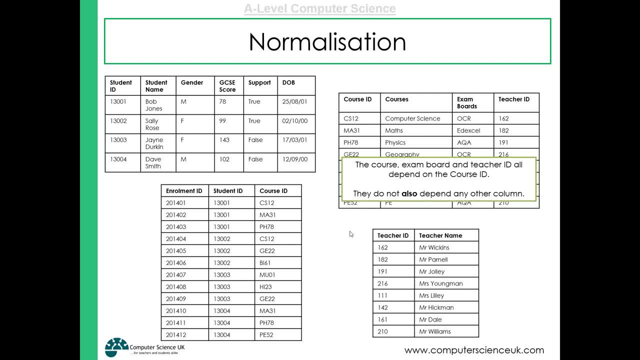 relational database. now, if we go through relational database, now, if we go through each one, the course, the exam board, the each one, the course, the exam board, the each one, the course, the exam board, the teacher ID, all depend on the course ID. teacher ID: all depend on the course ID. 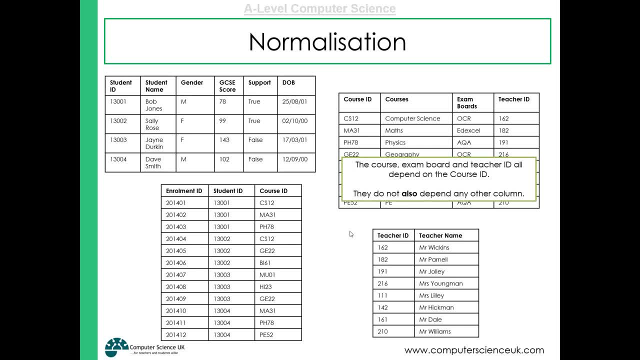 teacher ID. all depend on the course ID. they are also not also dependent on any. they are also not also dependent on any. they are also not also dependent on any other column. so the course computer, other column, so the course computer, other column, so the course computer science, the exam board, the teacher ID. 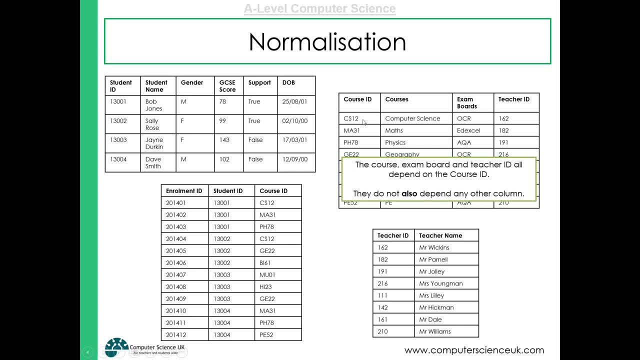 science, the exam board, the teacher ID, science, the exam board, the teacher ID. all of those are dependent on the course. all of those are dependent on the course. all of those are dependent on the course ID and they're not dependent on any ID and they're not dependent on any. 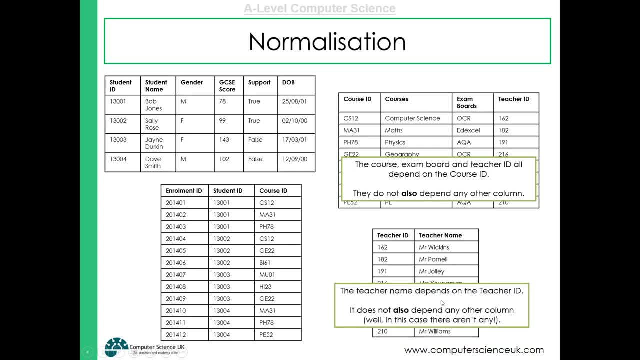 ID and they're not dependent on any other. so that's fine here the teacher other. so that's fine here the teacher other. so that's fine here the teacher name depends on the teacher ID. it does name depends on the teacher ID. it does name depends on the teacher ID. it does not also depend on any other column and 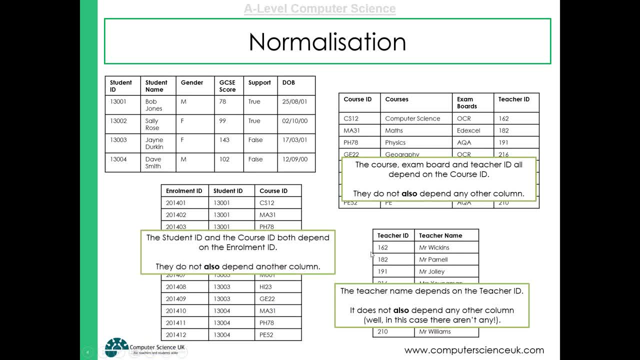 not also depend on any other column. and not also depend on any other column. and in this case there aren't any others. the in this case there aren't any others, the in this case there aren't any others. the student ID, the course ID: both depend on. 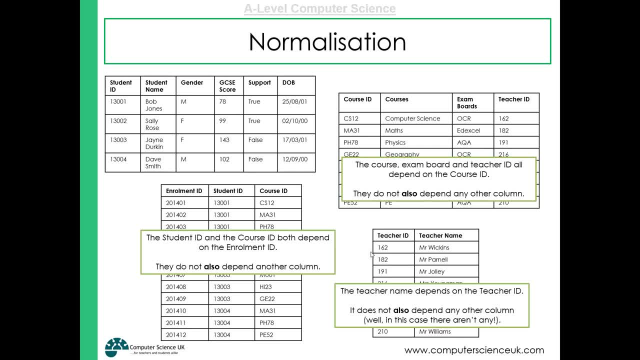 student ID, the course ID both depend on student ID. the course ID both depend on the enrollment ID. they do not depend on the enrollment ID. they do not depend on the enrollment ID. they do not depend on any other column. so that's also fine. but the enrollment ID, they do not depend on any other column, so that's also fine. but the enrollment ID. they do not depend on any other column, so that's also fine. but let's have a look at this and any other column, so that's also fine. but let's have a look at this and any other column, so that's also fine, but let's have a look at this and hopefully this is where the penny drops. 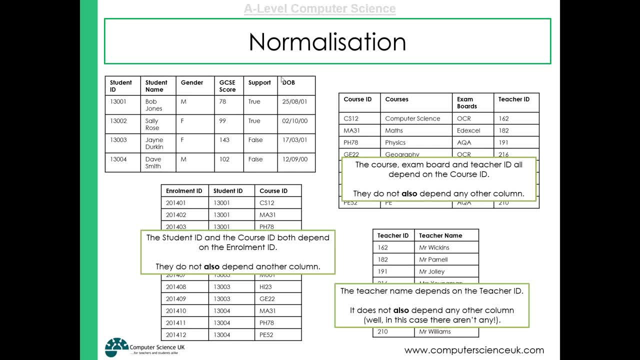 hopefully, this is where the penny drops. hopefully, this is where the penny drops when we are talking about third normal, when we are talking about third normal, when we are talking about third normal form in this table, here with our student form, in this table, here with our student. 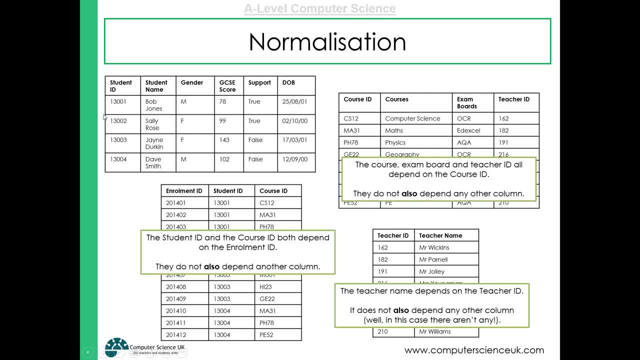 form in this table here with our student name, gender, GCSE score, support. date of name, gender GCSE score support. date of name, gender, GCSE score, support, date of birth says that the student name, the birth, says that the student name, the birth says that the student name, the gender, the GCSE score, support and date. 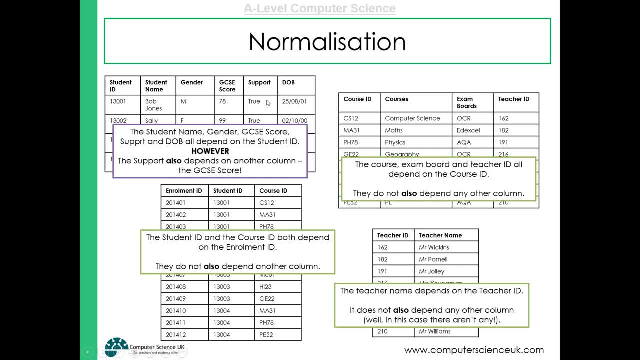 gender, the GCSE score, support and date: gender, the GCSE score, support and date of birth: all depend on the student ID of birth. all depend on the student ID of birth. all depend on the student ID. well, we know that it's in second normal. well, we know that it's in second normal. 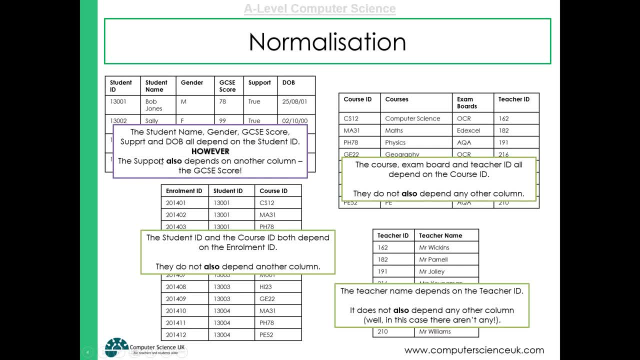 well, we know that it's in second normal form. however, support also depends on form. however, support also depends on form. however, support also depends on another column. support depends on their another column. support depends on their another column. support depends on their GCSE score: whether this student gets 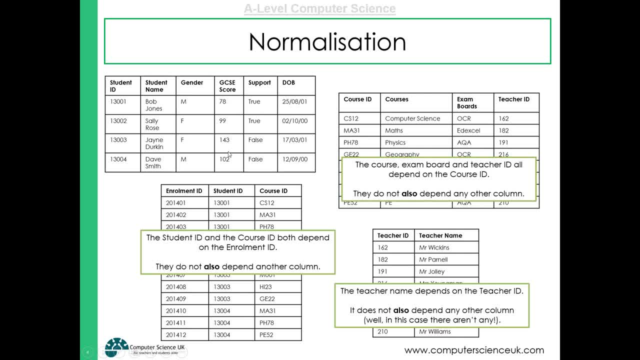 GCSE score. whether this student gets GCSE score, whether this student gets support or not, depends on the score. that support or not depends on the score. that support or not depends on the score that they got at GCSE in this case. if it's, they got at GCSE. in this case, if it's, 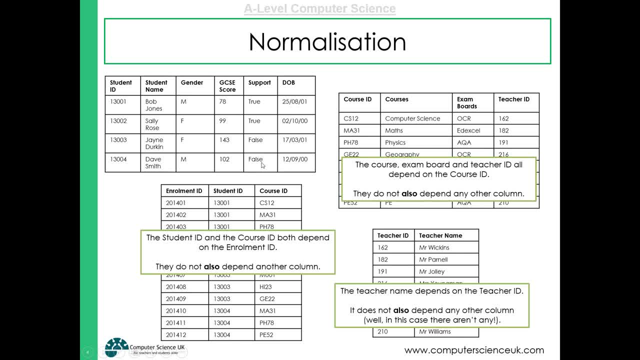 they got at GCSE. in this case, if it's less than 100, they need support. if it's less than 100, they need support. if it's less than 100, they need support. if it's more, they don't need support. so yes, more they don't need support, so yes. 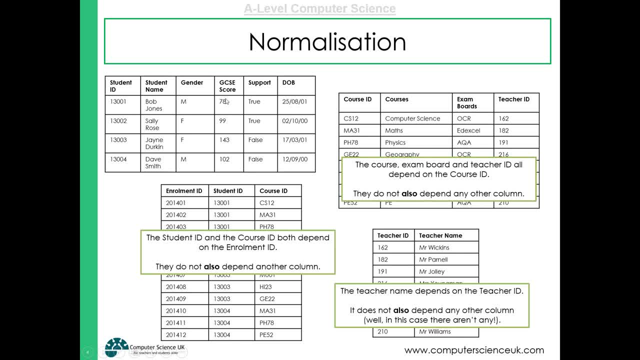 more. they don't need support. so, yes, support is dependent on the student. support is dependent on the student. support is dependent on the student. their GCSE score belongs to the student. their GCSE score belongs to the student. their GCSE score belongs to the student, so it's dependent on the student ID. the 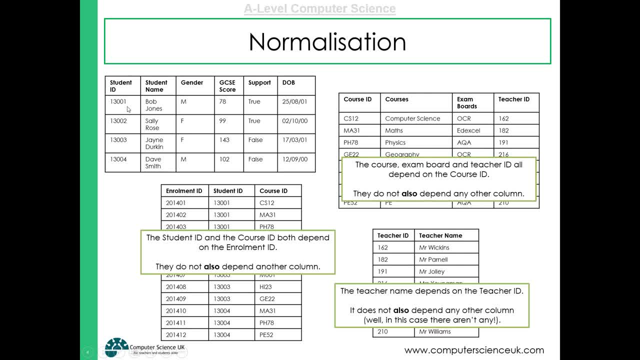 so it's dependent on the student ID. the, so it's dependent on the student ID. the date of birth, gender and their name: date of birth, gender and their name. date of birth, gender and their name: definitely all dependent on the student, definitely all dependent on the student. 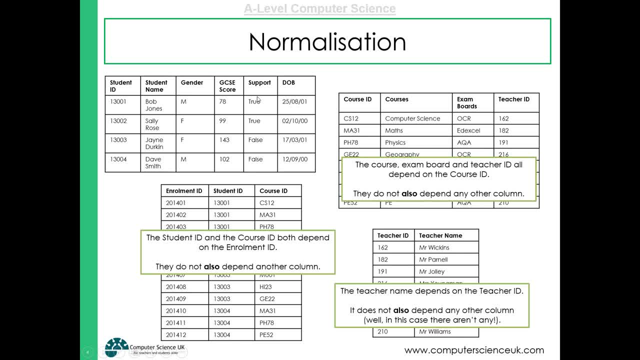 definitely all dependent on the student ID. they all relate just to the student ID. they all relate just to the student ID. they all relate just to the student ID. however, support also relates to GCSE ID. however, support also relates to GCSE ID. however, support also relates to GCSE score. so this is in second normal form. 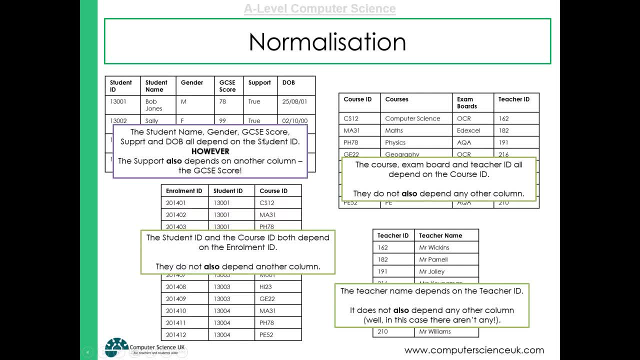 score. so this is in second normal form score. so this is in second normal form, but it's not yet in third normal form. but it's not yet in third normal form, but it's not yet in third normal form. so a database will be in third normal. 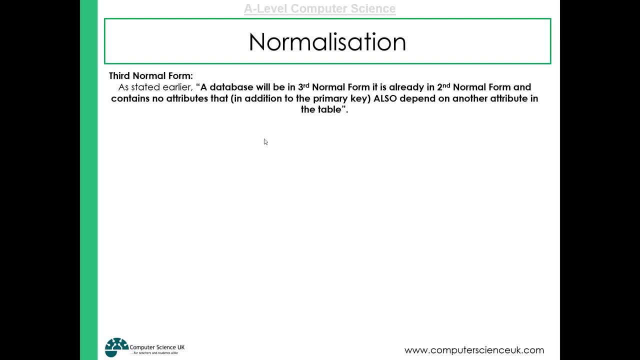 so a database will be in third normal. so a database will be in third normal form if it's already in second normal form. if it's already in second normal form. if it's already in second normal form and contains no attributes that in form and contains no attributes that in. 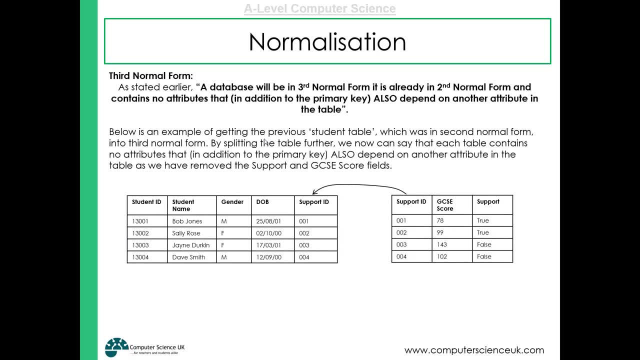 form and contains no attributes, that, in addition to the primary key, also depend. addition to the primary key also depend. addition to the primary key also depend on another attribute in the table. so on another attribute in the table, so on another attribute in the table. so here's an example of getting that. 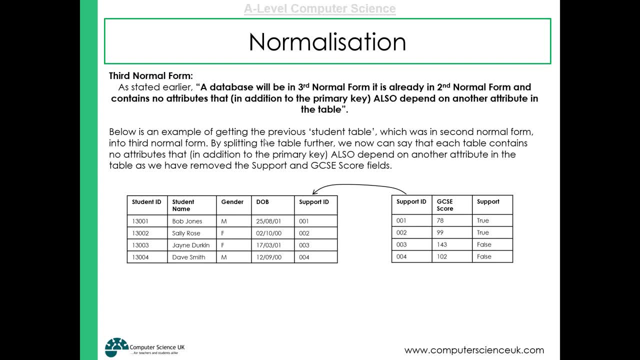 here's an example of getting that. here's an example of getting that previous student table that was in previous student table that was in previous student table that was in second normal form into third normal, second normal form, into third normal, second normal form, into third normal form. we split the table further and now 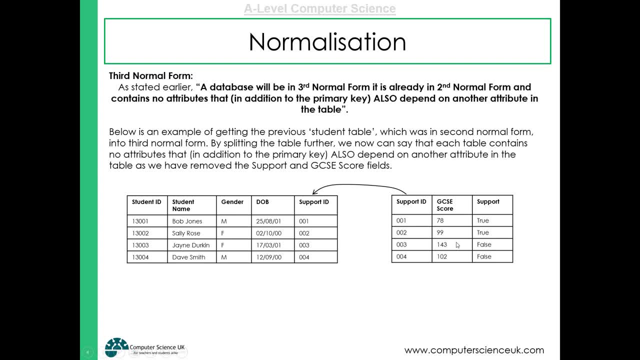 form, we split the table further and now form we split the table further and now we can see and say that each table we can see, and say that each table we can see and say that each table contains no attributes that, in addition, contains no attributes that, in addition, 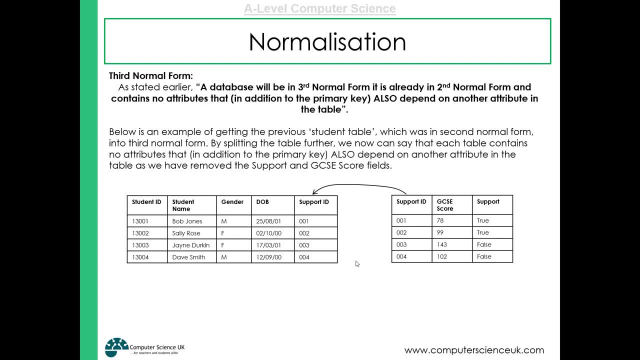 contains no attributes that, in addition to the primary key, also depend on to the primary key. also depend on to the primary key. also depend on another attribute in the table, as we've another attribute in the table. as we've another attribute in the table, as we've removed support and GCSE score fields, so 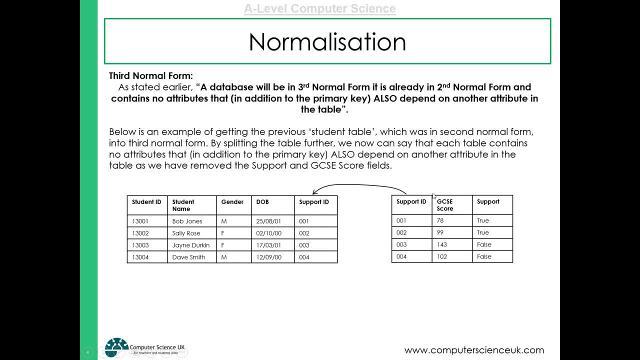 removed support and GCSE score fields. so removed support and GCSE score fields. so now, what we've got is our student table. now, what we've got is our student table. now, what we've got is our student table. we've got a support table, whether they 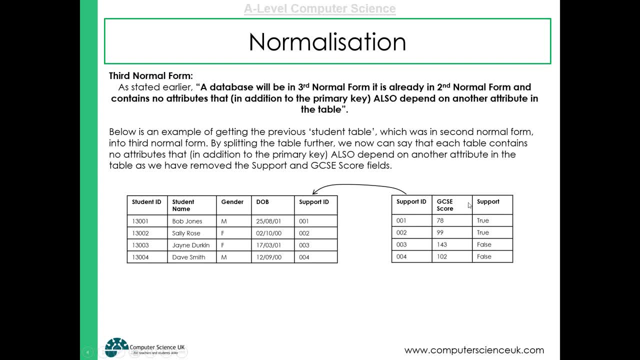 we've got a support table. whether they we've got a support table, whether they get support or not is dependent on the get. support or not is dependent on the get. support or not is dependent on the GCSE score. both of those things are GCSE score. both of those things are. 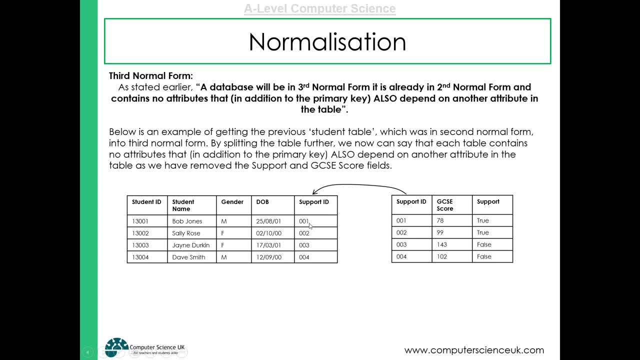 GCSE score. both of those things are dependent on the support ID, and then we dependent on the support ID, and then we dependent on the support ID, and then we can put the support ID into the student, can put the support ID into the student, can put the support ID into the student table. so our database is now in third. 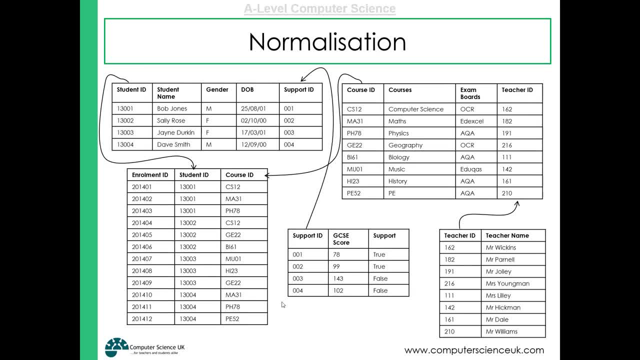 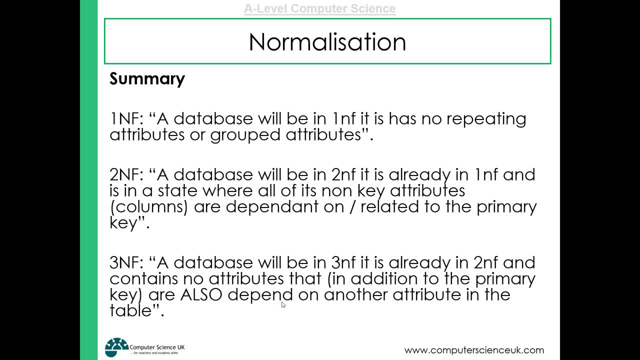 table. so our database is now in third table. so our database is now in third normal form. and here are the normal form and here are the normal form and here are the relationships. so in summary: first normal relationships. so in summary: first normal relationships. so in summary: first normal form. the database will be in first and 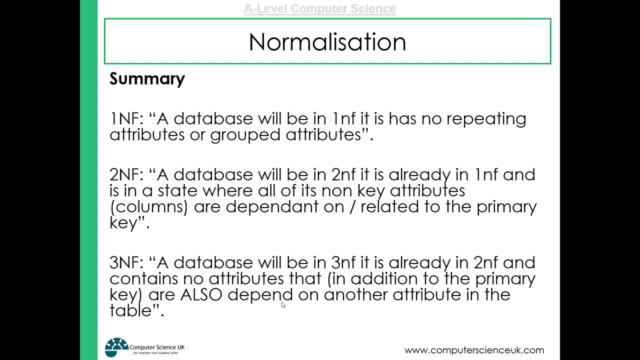 form. the database will be in first and form. the database will be in first and form if it's got no repeating attributes form. if it's got no repeating attributes form. if it's got no repeating attributes or grouped attributes, so getting that. or grouped attributes, so getting that. 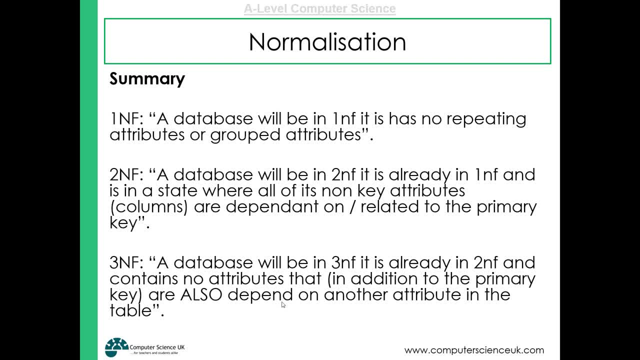 or grouped attributes. so getting that table into a flat file database with table into a flat file database with table into a flat file database with each record having no repeating each record, having no repeating each record, having no repeating attributes and no grouped attributes. attributes and no grouped attributes. 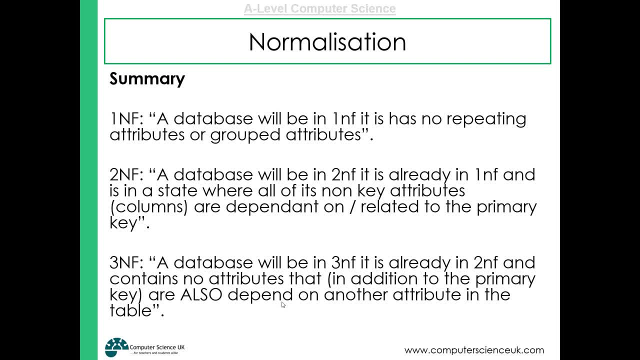 attributes and no grouped attributes, that's, that's the first step. if we want, that's, that's the first step. if we want, that's that's the first step. if we want to then go on to second normal form, it's to then go on to second normal form. it's. 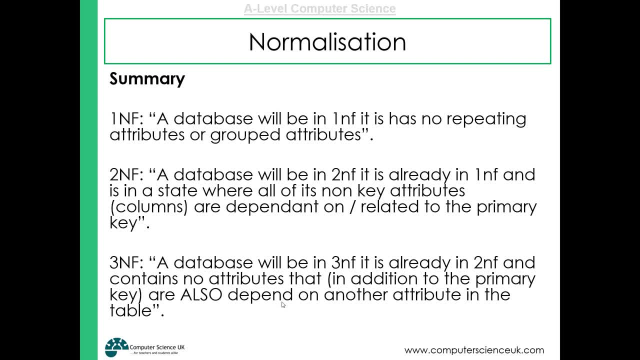 to then go on to second normal form. it's about making sure that we identify. what about making sure that we identify? what about making sure that we identify what the different entities are and split the the different entities are and split the the different entities are and split the database up into separate tables each. 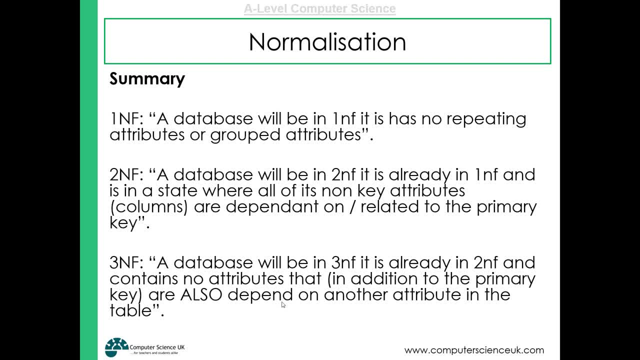 database up into separate tables, each database up into separate tables, each table being about an entity and then table being about an entity and then table being about an entity, and then. third, normal form is a very tricky step. third, normal form is a very tricky step. third, normal form is a very tricky step, whereby we look at each of those tables. 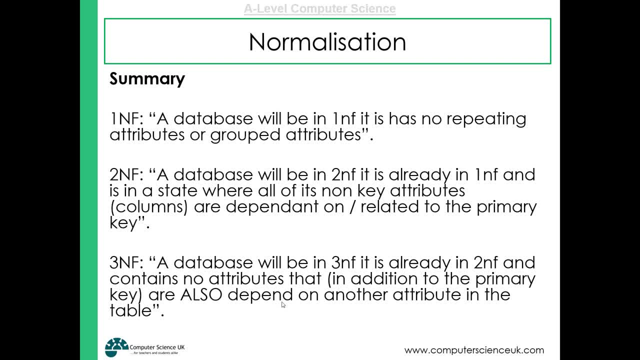 whereby we look at each of those tables, whereby we look at each of those tables that we've created in our relational, that we've created in our relational, that we've created in our relational database, and we ensure that each of database and we ensure that each of. 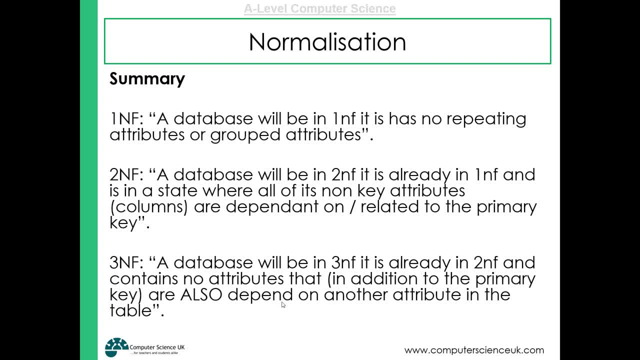 database and we ensure that each of those attributes that they don't in those attributes that they don't in those attributes that they don't, in addition to the primary key also depend. addition to the primary key also depend. addition to the primary key also depend on another actually in the table and if 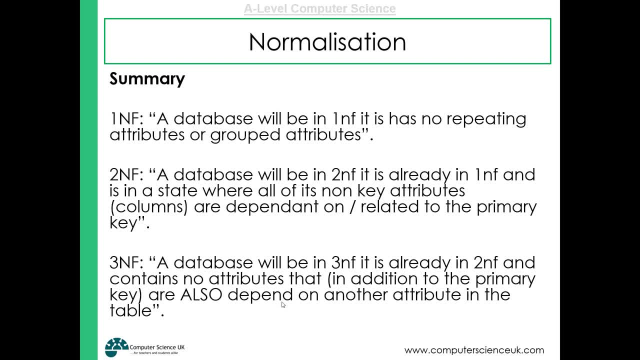 on another actually in the table and if on another actually in the table, and if they do, we split it up further.